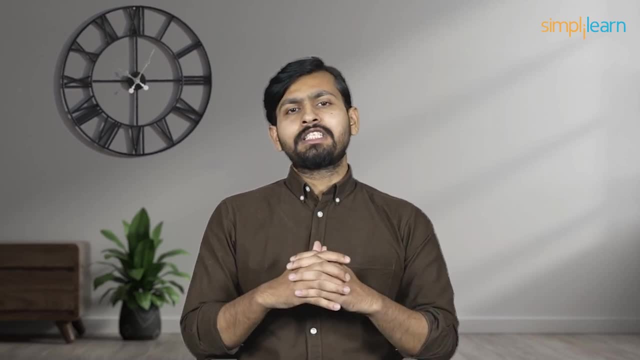 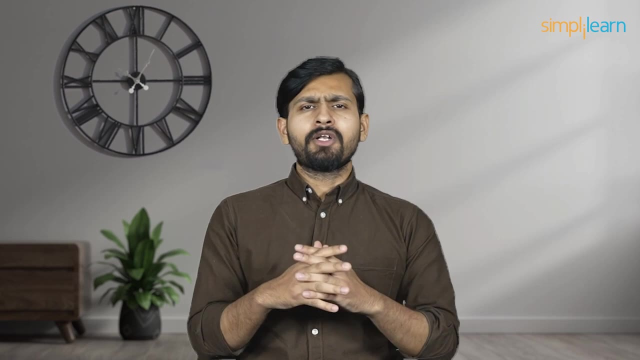 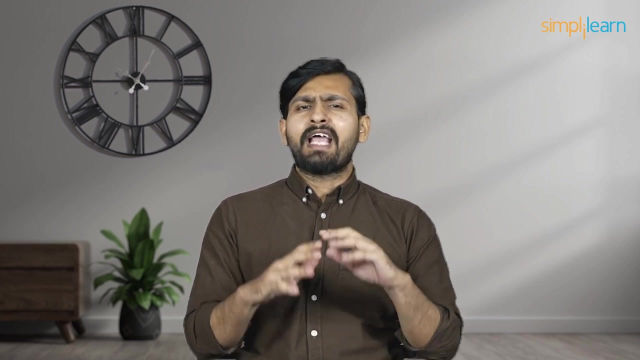 In today's fast-paced world, software development methodologies are continuously evolving to keep up the dynamic nature of the technology and the market demands. Agile methodologies has emerged as a leading approach in software engineering, transforming traditional development practices, with emphasis on flexibility, collaboration and iterative energy. In this tutorial, we will delve. 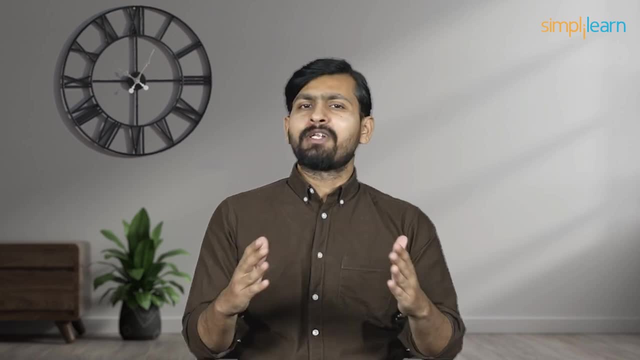 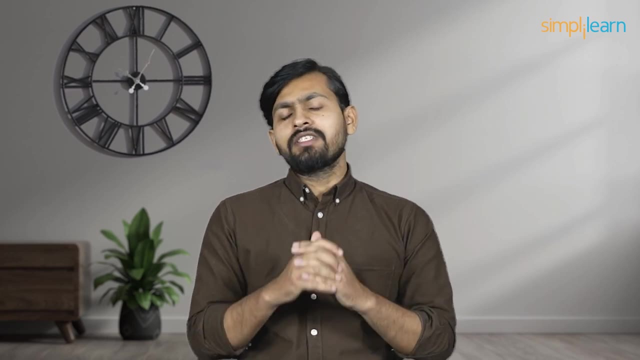 into the agile model in software engineering, exploring its principles, benefits, common frameworks, implementation strategies and challenges. So guys watch this video till the end if you want to learn more about agile principles, and I request you guys that do not forget to hit. 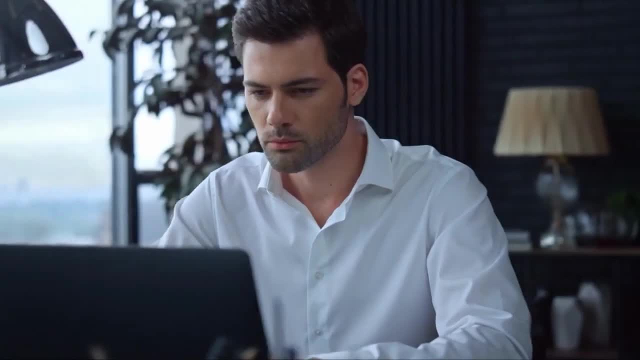 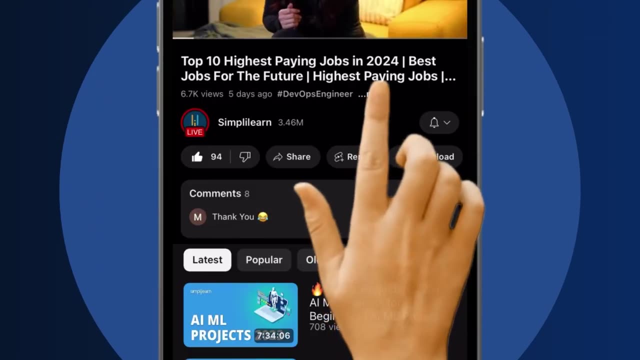 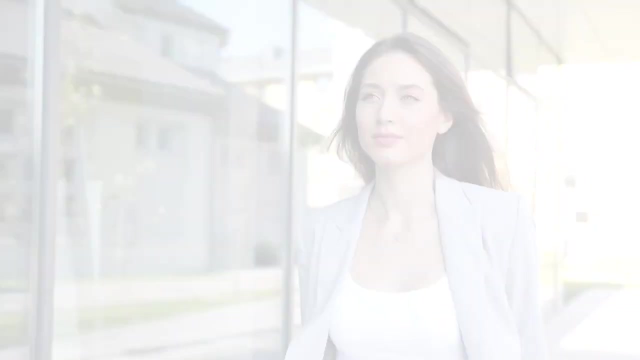 the subscribe button and click the bell icon for the further updates. Craving a career upgrade? Subscribe, like and comment below. Dive into the link in the description to fast track your ambitions, Whether you're making a switch or aiming higher. SimplyLearn has your back. 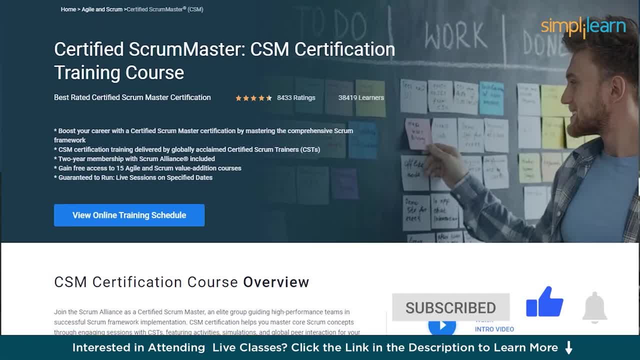 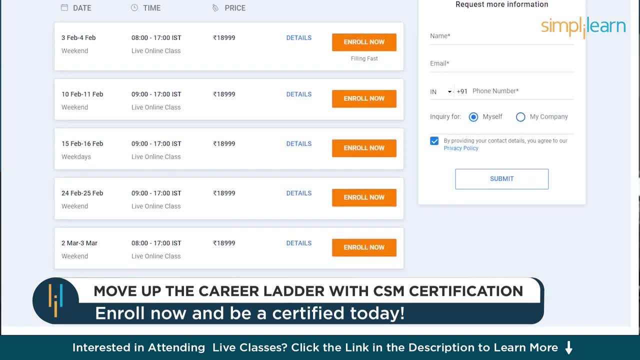 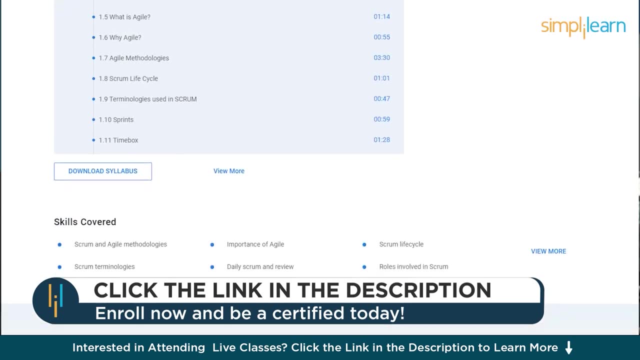 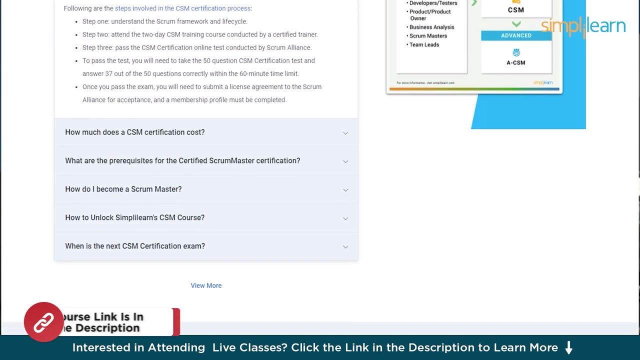 SimplyLearn has got certified scrum master certification course. In this course you're going to learn about scrum concepts through engaging session with the CSTs, featuring activities, simulations, global PRA interactions for your scrum master certification. Hurry up, guys, join the course now. The course link is given in the description box. 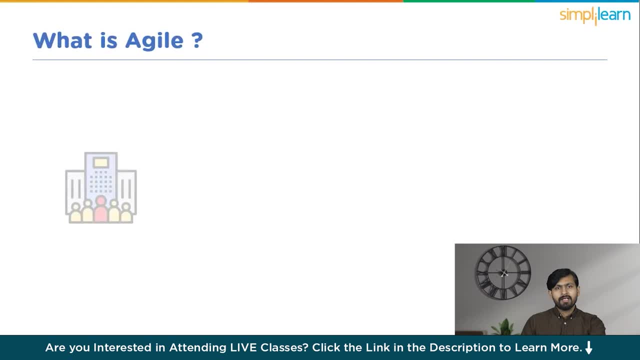 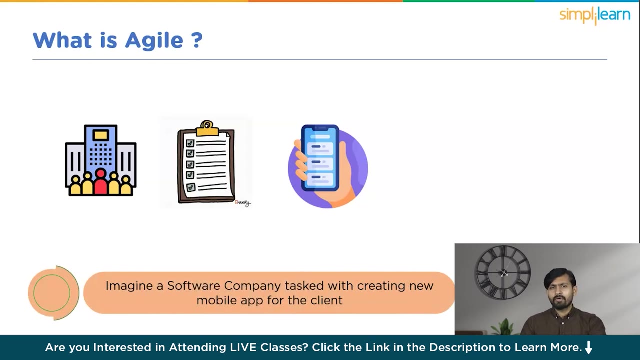 So, guys, let's start with what is agile. So, guys, imagine a software development company tasked with creating a new mobile app for the client. Using agile methodologies, the development team breaks down the project into smaller iterations or sprints, each focused on delivering specific features or functionalities. 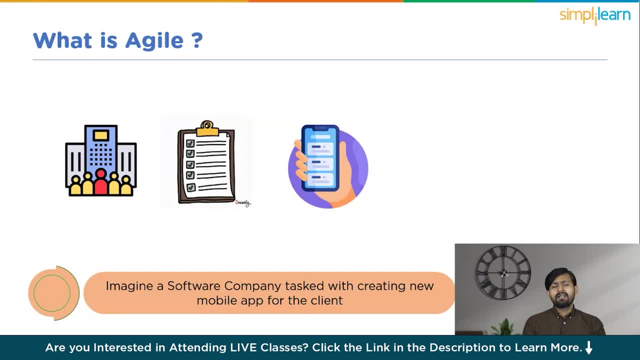 During each sprint, the team collaborates closely with the client to gather feedback, prioritize features and make necessary adjustments. They work in short cycles, typically two to four weeks, delivering incremental updates to the app. Now you'll be wondering, but what's the technical definition of agile principle? is? 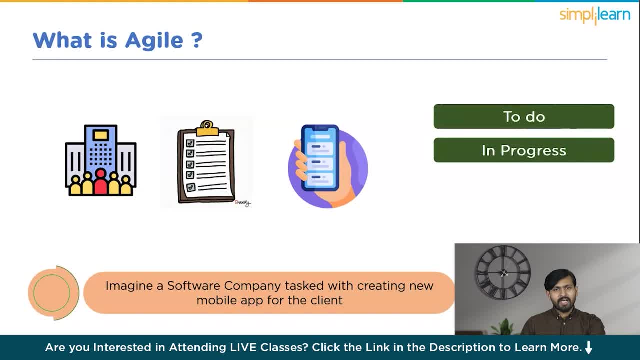 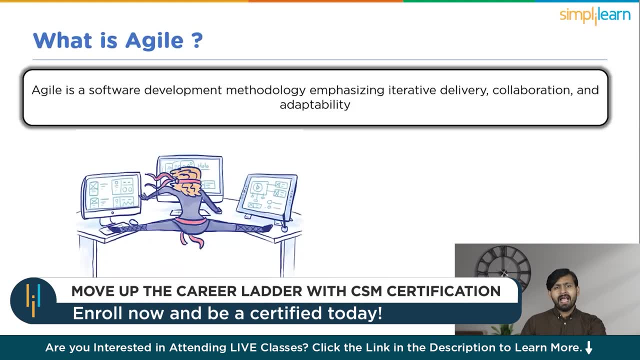 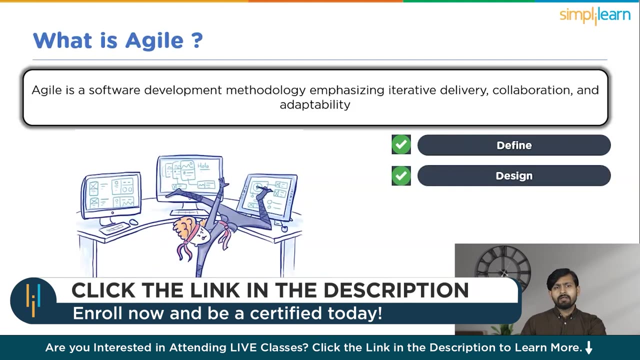 Now let's move on and discuss the technical definition of agile. So guys, agile is a software development methodology emphasizing iterative delivery, collaboration and adaptability. It prioritizes satisfaction through frequent delivery of valuable software increments, promoting close collaboration between cross-functional teams and stakeholders. Agile fosters flexibility by embracing 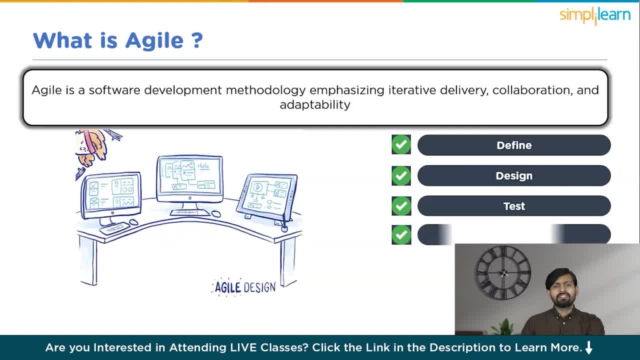 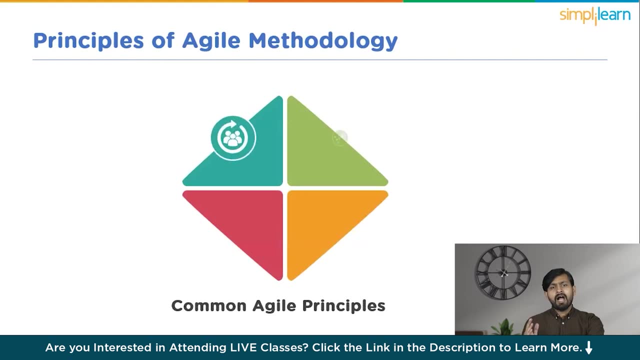 changing requirements and encourages self-organization and continuous improvement within the development team. Now, guys, let's move on and discuss some of the core principles of the agile methodology. So, guys, at its core, agile methodologies is guided by a set of principles outlined in the Agile Manifesto, a foundational document which 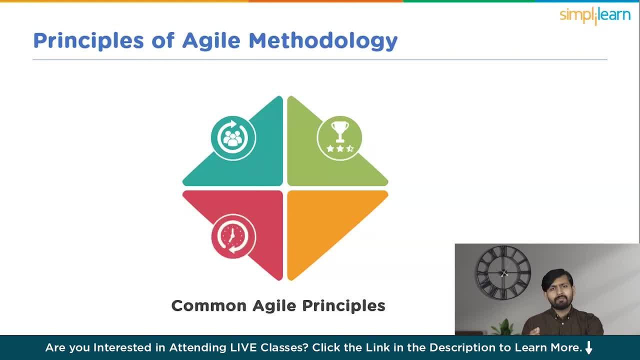 was created by a group of software developers in 2001.. And these principles include the first one, that is, individual and interaction over processes and tools. Agile places a strong emphasis on human aspect of software development, prioritizing effective communication, collaboration and teamwork within the development team. 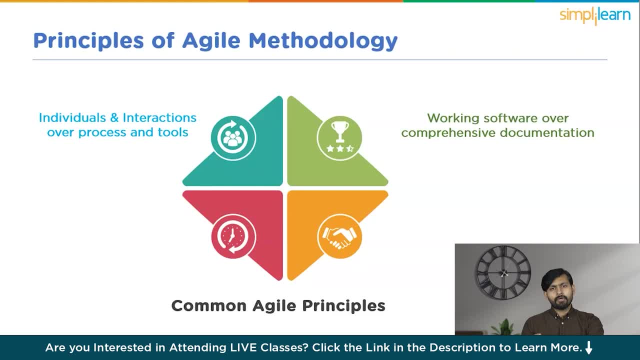 The next one is working software over comprehensive documentation. Well, as we all know that documentation is important, but agile prioritizes the delivery of functional software. It emphasizes the value of tangible outcomes over the extensive documentation, ensuring that the software meets the needs of stakeholders. The next principle is customer collaboration over contract negotiation. 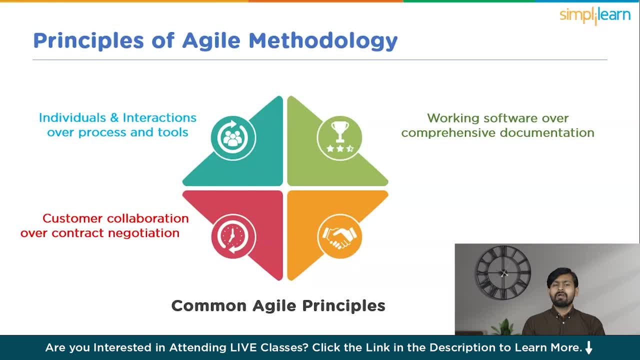 Agile encourages close collaborations with customers or stakeholders throughout the development process. By involving customers in the decision-making process, agile ensures that the software solutions align with user requirements and also expectations. Next one is responding to change over following a plan. Agile acknowledges the inevitability of changes in the software. 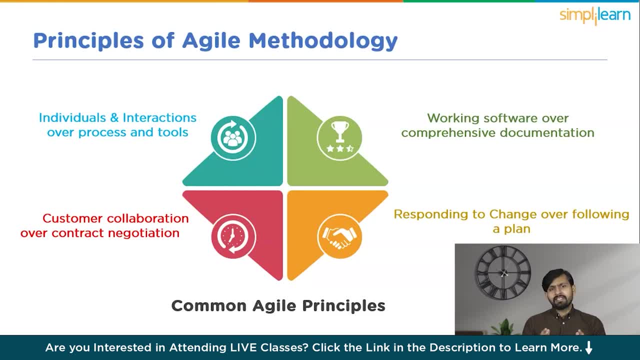 development projects. It promotes adaptability and flexibility, allowing teams to respond quickly to changing requirements and priorities. This principle forms the foundation of agile principles and shaping the way software development teams approach their work and also interact with the stakeholders. Now we will move on and discuss the benefits of using agile methodologies. 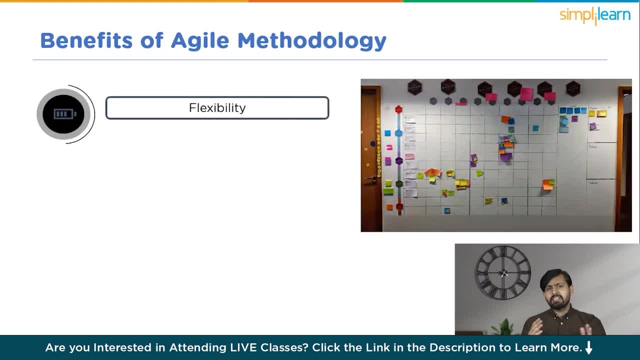 Agile methodology offers several benefits over the traditional waterfall models. The first one is flexibility. Agile methodology enables teams to adapt to changing requirements and also market conditions very quickly By breaking projects into smaller iterations. agile allows for continuous refinement and adjustment, ensuring that the software solutions 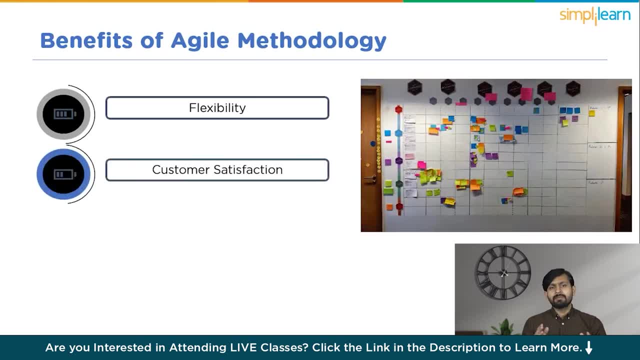 remain relevant and responsive. The next one is customer satisfaction. Agile's focus on customer satisfaction and frequent delivery of working software leads to a higher level of customer satisfaction. By involving customers throughout the development process, agile ensures that the software solution meets the user needs effectively. Next one is faster time to market Agile iterative. 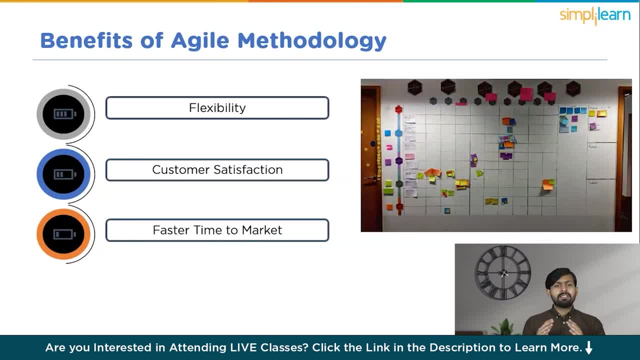 approach to development enables a team to deliver software in small and incremental releases. This results in faster time to market, allowing organizations to respond to market demands and also user feedback more rapidly. So, guys, the next one is enhanced collaboration. Agile fosters a collaborative working environment where team members work very closely together. 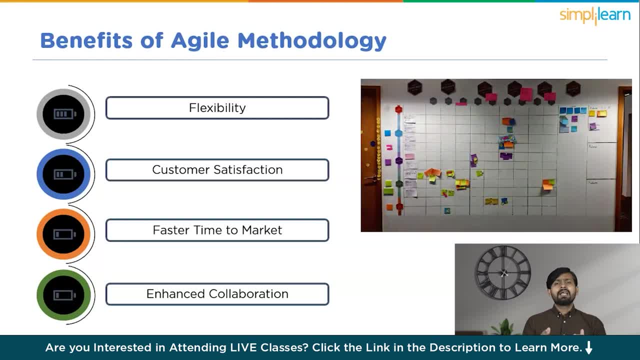 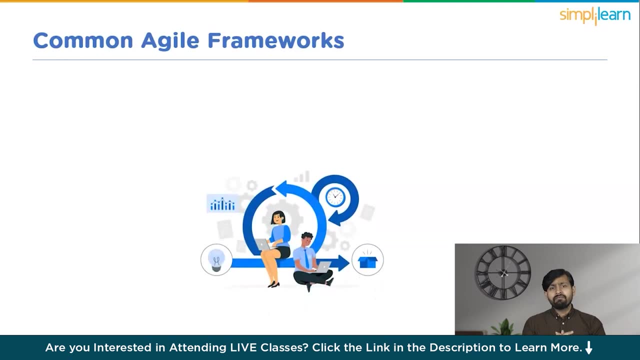 to achieve common goals. by promoting transparency, communication and shared responsibility, Agile improves team morale and also productivity. Now let us discuss some of the common agile frameworks that are used in the software development industry. So there are several common agile frameworks and methodologies, each offering its own approach to implementing agile principles. 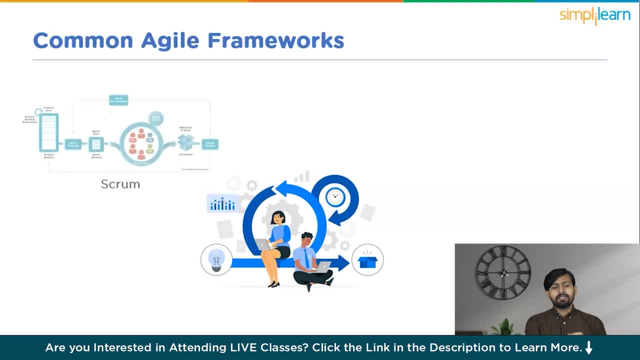 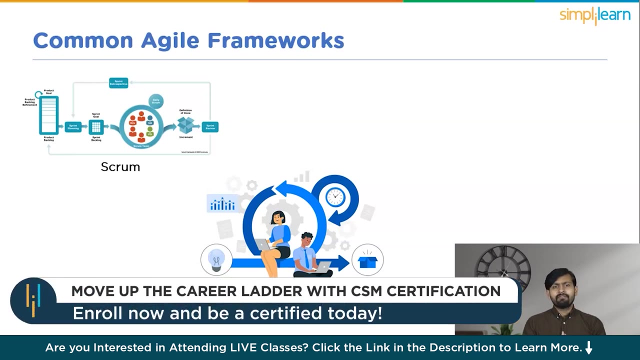 effectively. Some of the widely used frameworks include Scrum, which is a popular agile framework characterized by its iterative approach to development and its emphasis on self-organizing cross-functional teams. Scrum teams work, in short, iterations, called sprints, delivering incremental releases of working software. Next we have is Kanban. Kanban is a 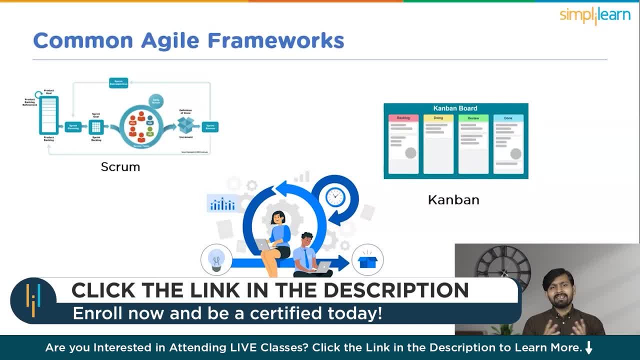 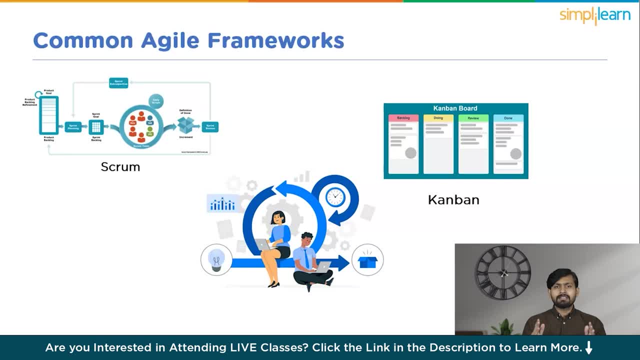 framework that focuses on workflow optimization and continuous delivery. Kanban boards are used to visualize in progress, allowing teams to identify bottlenecks and also optimize their process accordingly. Next we have all over here is extreme programming. Extreme programming is agile framework that emphasizes engineering practices such as test-driven development, peer programming. 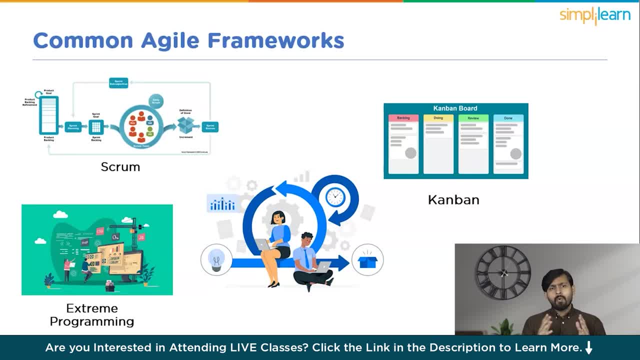 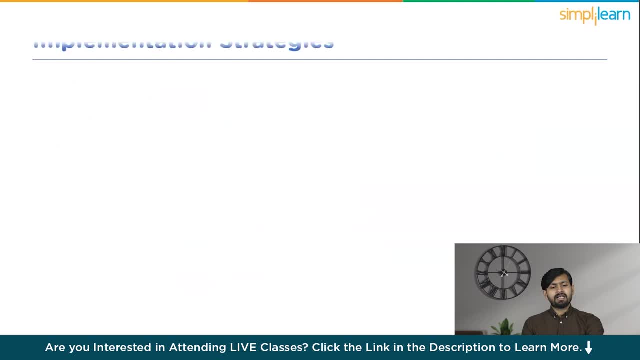 and continuous integration. Extreme programming team works collaboratively to deliver high-quality software quickly and efficiently. Now we will move on and discuss about implementation strategies. So, guys, implementing agile methodologies successfully requires planning and execution. Some of the key strategies for implementing agile includes training and education: Providing training and education to team members to ensure 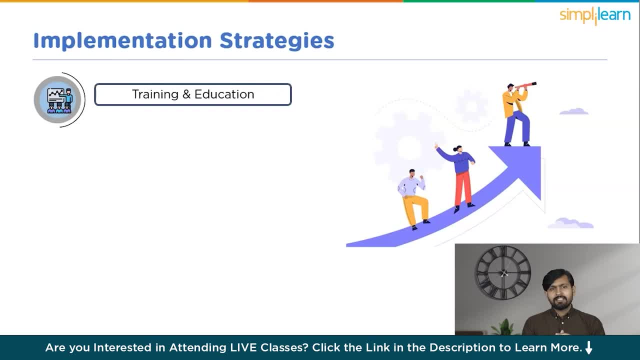 they understand agile principles and practices. This may include workshops, seminars and presentations to ensure that teams have necessary skills and knowledge to work effectively in an agile environment. Next we have all over here is cross-functional teams From cross-functional teams with members from different disciplines, such as development, testing and design. Cross 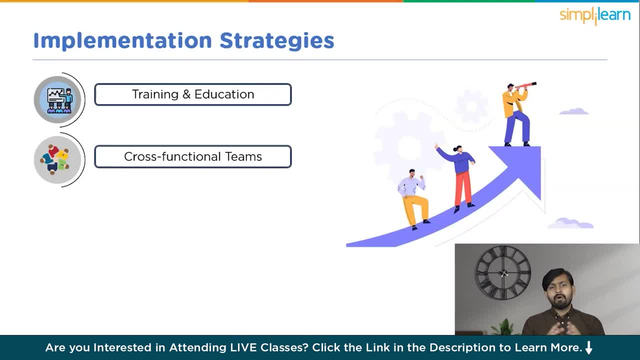 functional teams, promote collaboration and also ensures that all necessary skills are represented on the team, enabling teams to deliver high-quality software solutions more effectively. Next we have all over here is iterative approach: Adopting an iterative approach to development, breaking projects down into small and manageable chunks by delivering software in small increments. 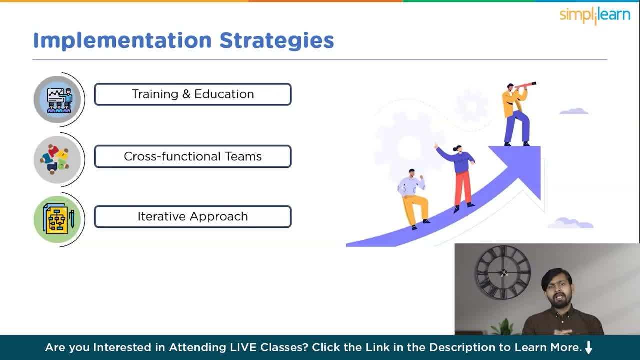 teams can get the feedback early and often allowing them to adjust their approach and deliver value to customers more effectively. Next, we have continuous improvement: Fostering a culture of continuous improvement within the organization, where teams are encouraged to experiment, learn from their mistakes and also make adjustments as needed. 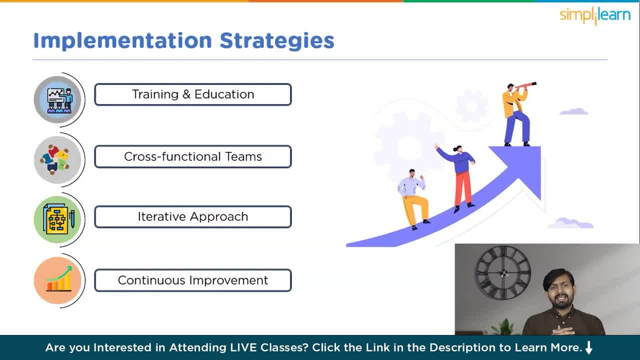 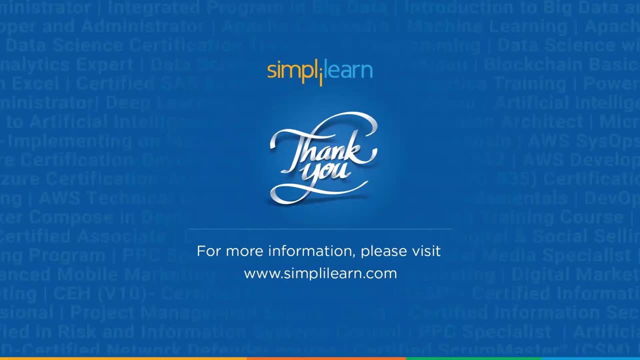 By promoting a culture of continuous improvement, organizations can adapt to changing market conditions and also deliver better software solutions more effectively. So, guys, these were some of the strategies that we have discussed that how we can implement this in agile principles. Thank you, guys, for watching this video on agile principles in software development. 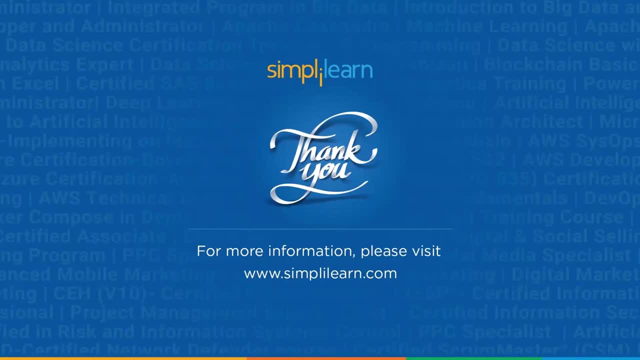 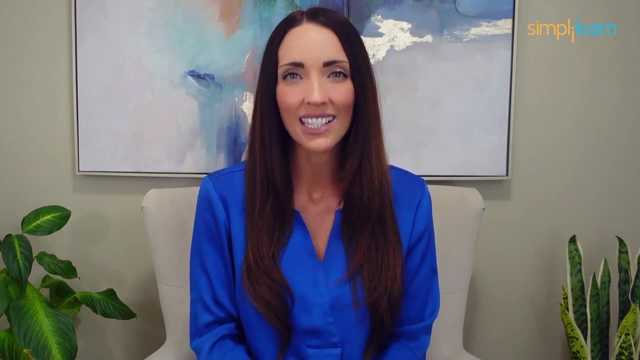 I hope so. you would have enjoyed our today's video. Thank you for watching. stay safe and keep learning. Staying ahead in your career requires continuous learning and skilling, Whether you're a student aiming to learn today's top skills, or a working professional. 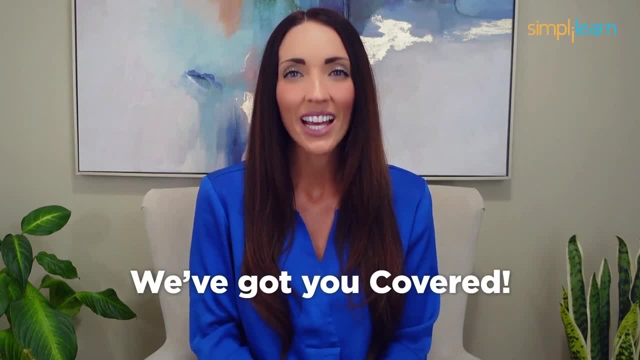 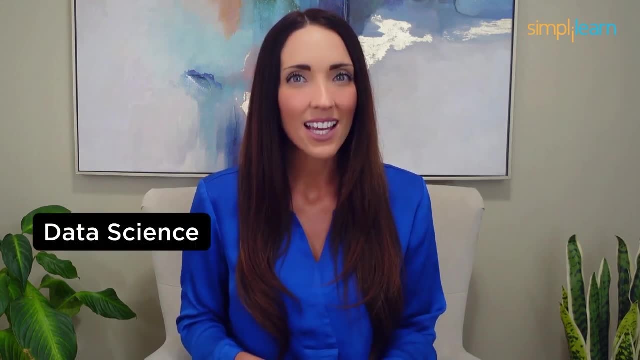 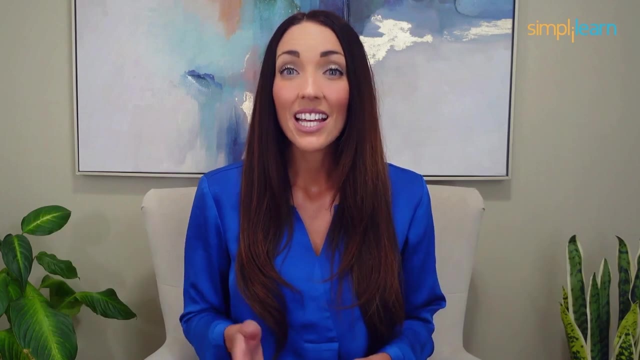